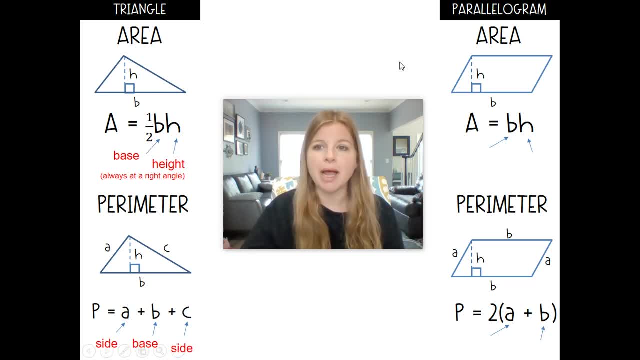 maybe with one of those special triangle rules. A parallelogram is basically two triangles together. So if the area formula for a triangle is one half base times height and I take a triangle and I simply double it, well, one half times two is one, And so the formula is just base times height, and it's the same exact idea I have. 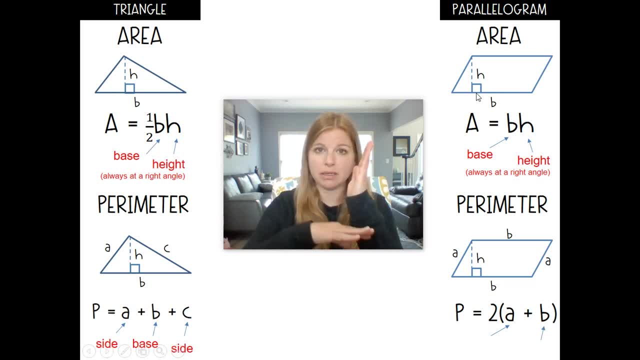 my base and my height is always at a perpendicular 90 degree angle and those would be the values and I just simply multiply them kind of like the rectangle formula: Times width, Parallelogram is base times, height. Notice, I don't care about like the slanted sides. 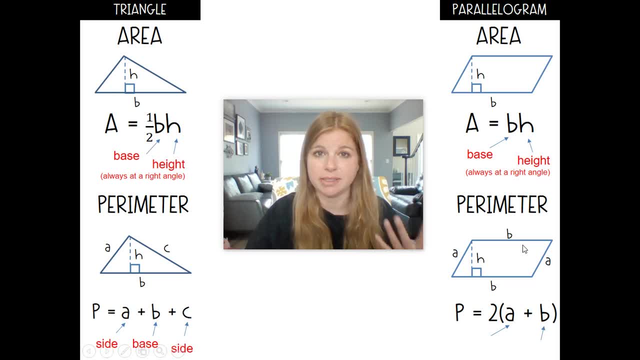 However, for the perimeter perimeter I wouldn't care about the height the same way as before. Maybe I need it, though. to find a certain side length I would simply add up my two different sides and then multiply it by two. I mean, I could do A plus B plus A plus B, but two times A plus B. 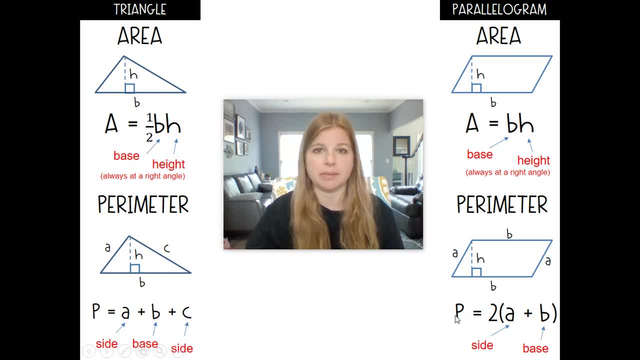 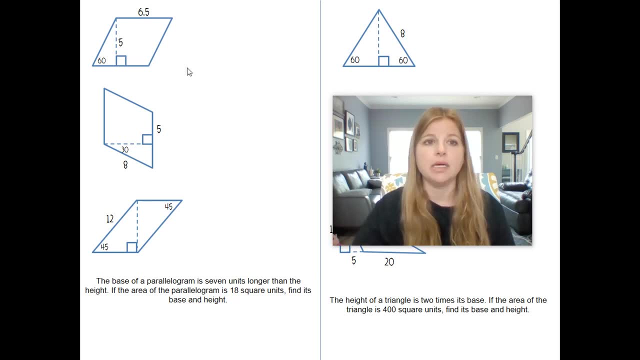 is the same thing. So two times the side and then two times the bases. Let's take a look at the next formula. Let's take a look at the parallelograms here on the left hand side. So here I'm given this parallelogram and I want to find the area and the perimeter of it. And, guys, all of our final. 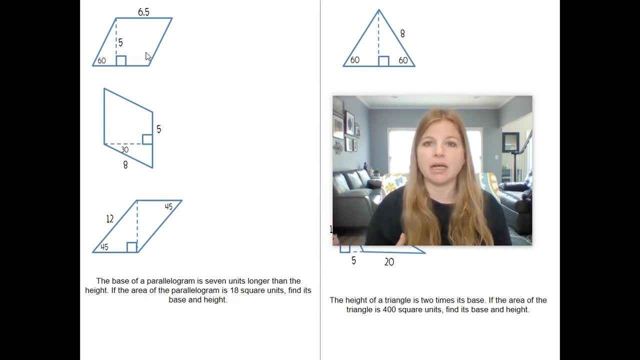 answers, we're going to round to the tenths place, but while we're doing some of the calculations we're going to round to the thousandths place. I generally always go out three place values until I get to my final answer, just so I can try to stay as accurate as possible. So here I have: a height. 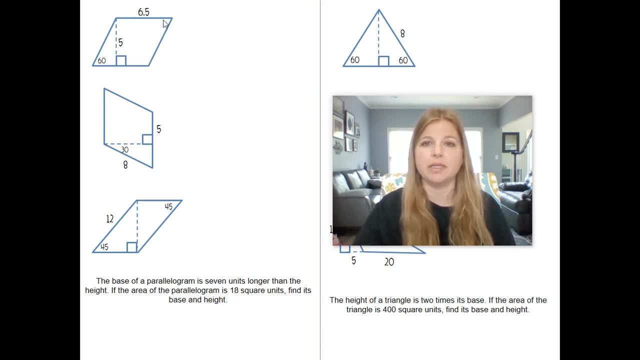 of five and I have a base of 6.5.. Remember, the base doesn't have to be at the bottom, It's simply where the height is perpendicular to the base. So here I would be able to just simply do the area which is five times 6.5,. 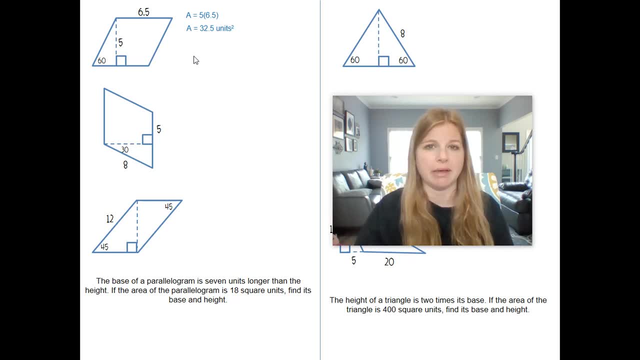 and I would get an area of 32.5 units, Some basic calculator work. But now if I wanted to calculate the perimeter, the problem is, I know that this length is 6.5 and so is this length, But I don't. 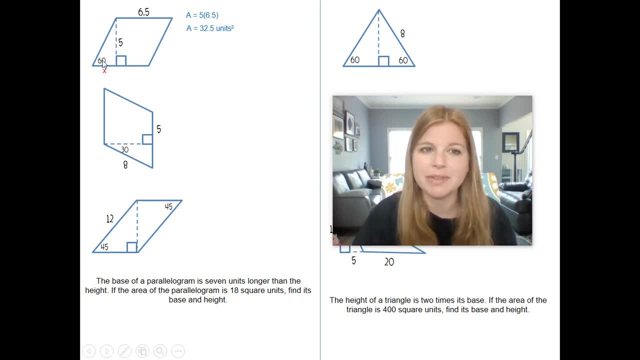 know what the left and right hand side of my parallelogram is, but I'm given this little symbol that there's a 60. So if I know that the side opposite the 60 is 5, remember your 30-60-90 rules, the side opposite. 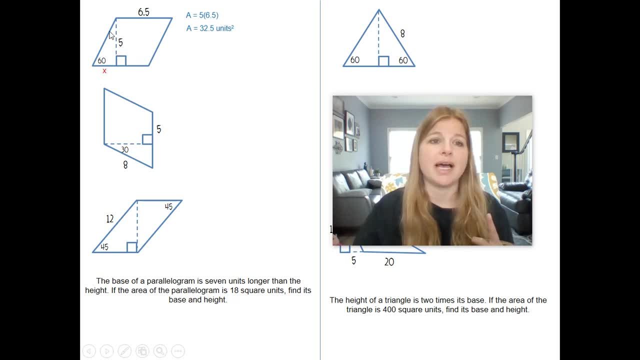 the 5 is the side opposite the 30,, which is x multiplied by radical 3.. So if I'm given the side opposite the 60,, in order to go to the side opposite the 30,, I need to take this 5 and divide. 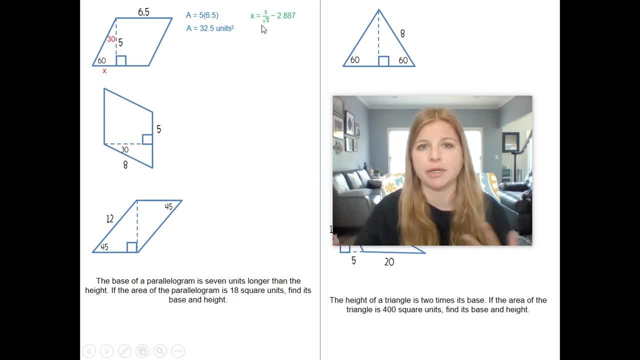 it by radical 3.. Now, I'm not going to rationalize the denominator and use my radicals Again. I'm going to put it in my calculator. I'm going to put it in my calculator and see where it gives me to the thousands place And that's. 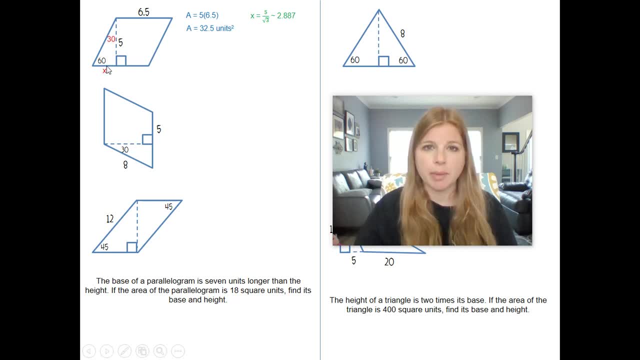 actually the length for x. And then remember the side opposite, the 30, with relationship to this side of this triangle, which is really the hypotenuse, is we double it So to find the hypotenuse of this little right triangle here, it would be two times that amount, which is 5.774.. 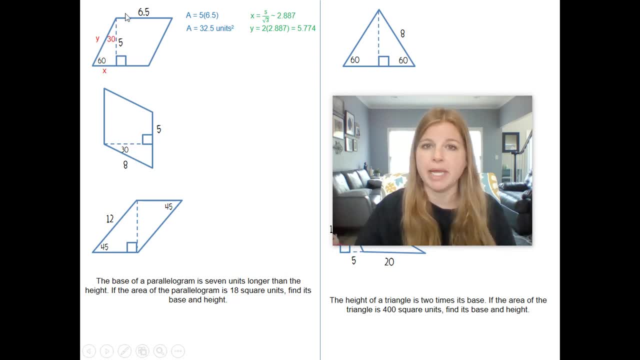 Now, I know the length of this side, I know the base. I simply do two times the sum of those terms. Or again, I could really just write 6.5 plus 6.5,, 5.774 plus 5.774, and rounding to the: 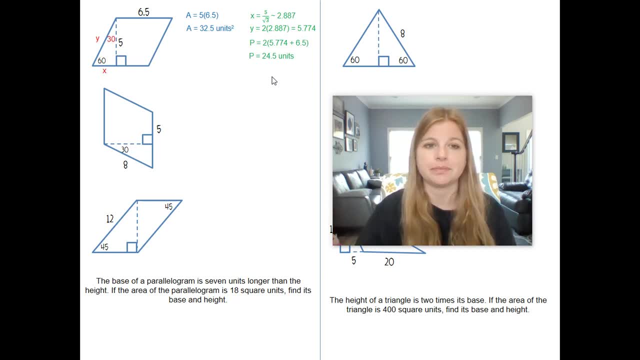 tens place for my final answer, I get 24.5.. Next one: I know that this little part here is 5.. I don't know this part. I do know the full length of this part of my parallelogram is 8, but I don't know the height and I don't know the full base. 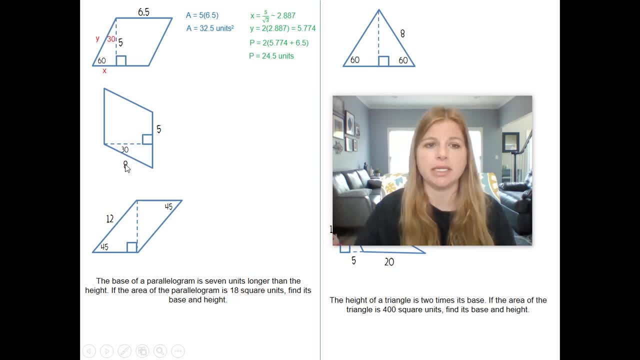 So I do know this is 30. And in this little right triangle here, this here 8, would be the hypotenuse. The relationship with the hypotenuse inside opposite the 30 is that side x is half of it. So if this length is 8,, then this length is 4.. Okay, so now I want to know the height. Well, 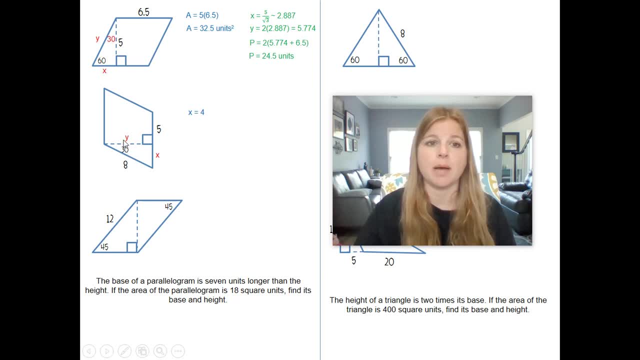 there's a couple ways I could do this. I could do the Pythagorean theorem. It would be this: y squared plus 4 squared equals 8 squared. Or, since it's a 30,, 60,, 90, I can know that the 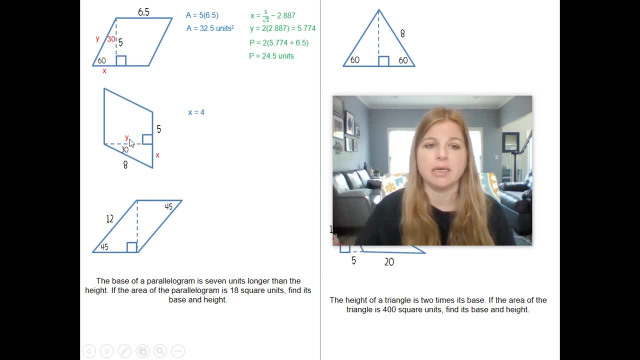 relationship between the side opposite the 30 to the side opposite the 60 is to multiply by radical 3.. So I do 4 times radical 3,, which is 6.928, which is my base now, or my height rather, excuse me. 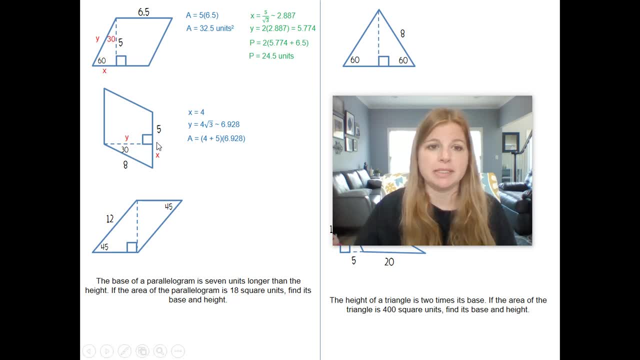 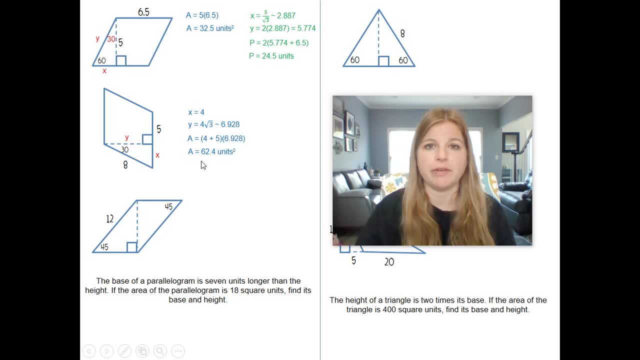 my height and I would get 62.4 units squared Parameter. well, since I know that this is 9 and this is 8, I would add those up and double it and I get 34 units. So again, this 9 is coming from the. 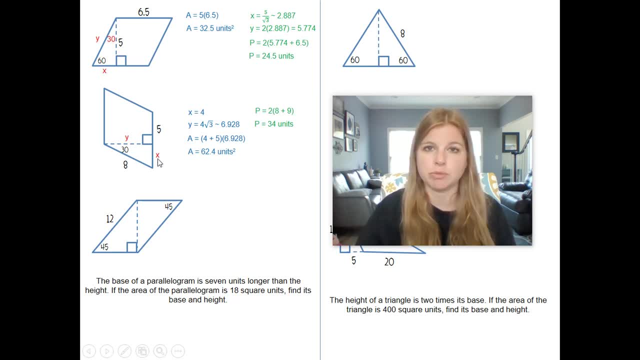 fact that we knew this was 5.. This little segment we saw, 4x, which was 4.. So altogether that whole side length is 9.. Next one: 45,, 45,, 90 triangles are built into this parallelogram. I have a. 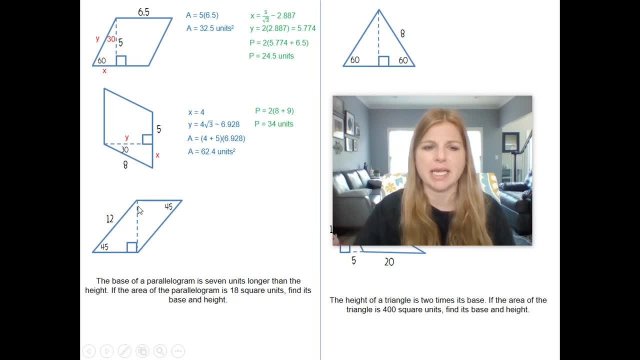 slant. but it's not my base. I need to know this base and this height: 45,, 45,, 90, we know those are isosceles triangles, So if I find x the height, it's also going to be the same height. 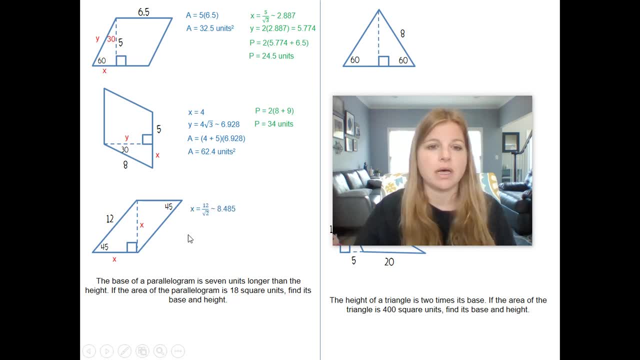 for my b, the same length for my base. So going from the hypotenuse to a side length, remember, is dividing by radical 2.. If I do 12 divided by radical 2, that means x is 8.485.. 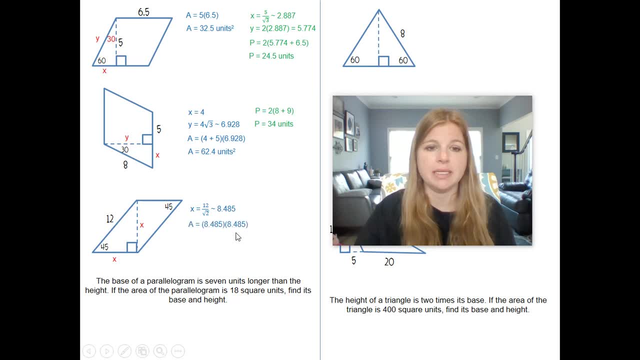 If I take that now, base times height, so they're both the same and you get 72 units squared Perimeter. this is 12, so it's this opposite side, and then I know that this side here is 8.485,. 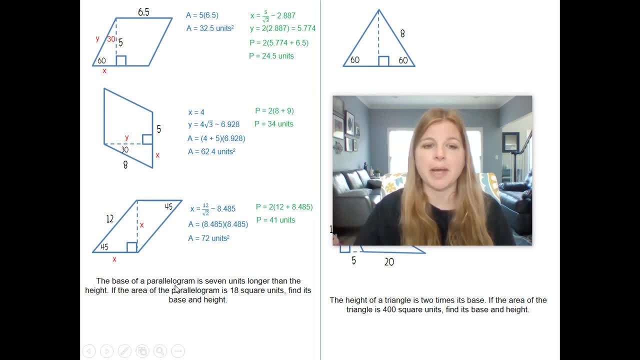 and my full perimeter is 41 units. The base of a parallelogram is 7 units longer than the height. If the area of the parallelogram is 18 square units, find its base and height Okay. So base of a parallelogram is 7 units longer than the height, So I'm going to call the height h. 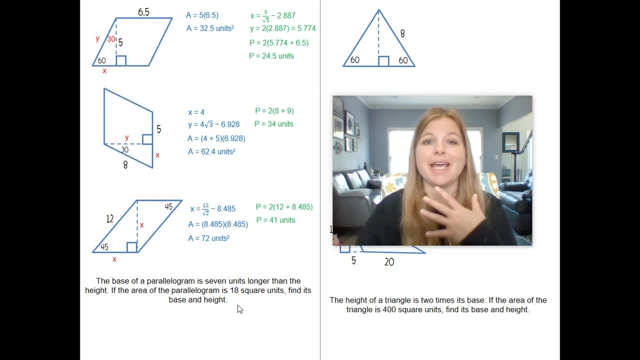 and then the base would be- I'm sorry- x, and then the base would be x plus 7. And if I multiply those together- the height and the base- that should be equal to 18.. Okay, so my area is equal. 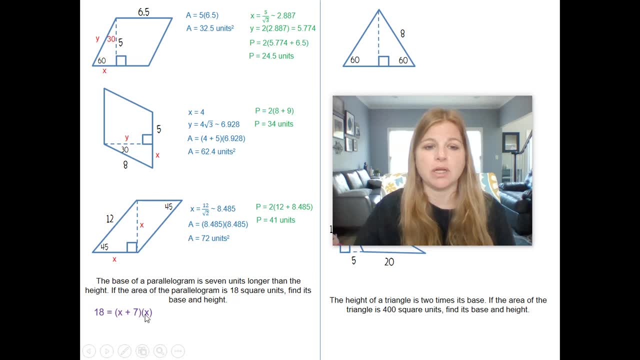 to the base of the parallelogram which is 7 units longer than the height. If I multiply this out, I get 18 equals x squared plus 7x. First step in solving a polynomial is to find the base of a parallelogram which is 7 units longer than the height. 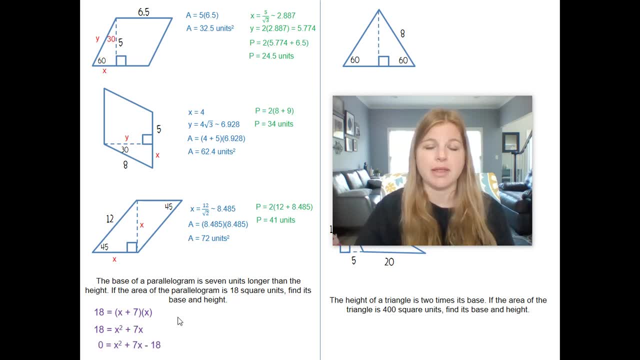 If I multiply this out, I get 18 equals x squared plus 7x. First step in solving a polynomial equation: set the equation equal to 0. Then we factor what factor pair of negative 18 gets you 7.. It's a positive 9 and a negative 2. Set each of those equal to 0, we get our two solutions of. 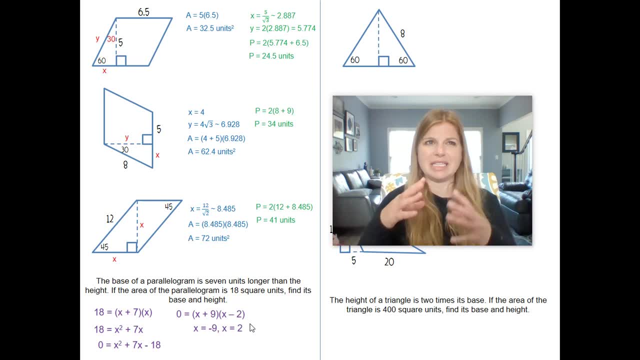 negative 9 and 2.. But think about it: Negative could never be an answer if, when you substitute it in, you get a negative length, And here I can't have a length of negative 9 and then double it and have another side of. let's say: 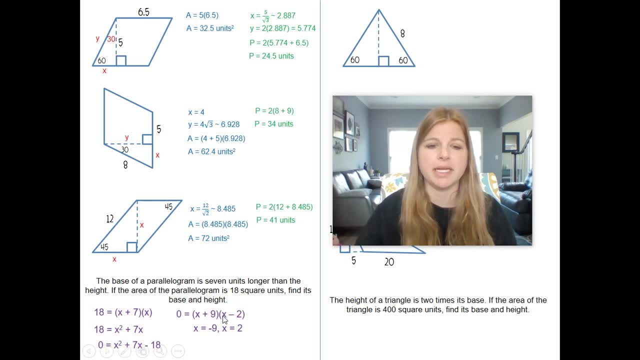 I'm sorry, add 7 to it, I'd still be in the negative. So the negative 9 is actually not part of the solution. So this means it says the base of a parallelogram is 7 units longer than the height. So that means that x is the height, so the height is 2, and the base would have to be: 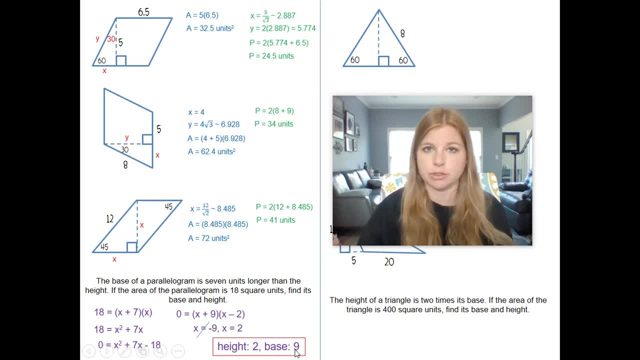 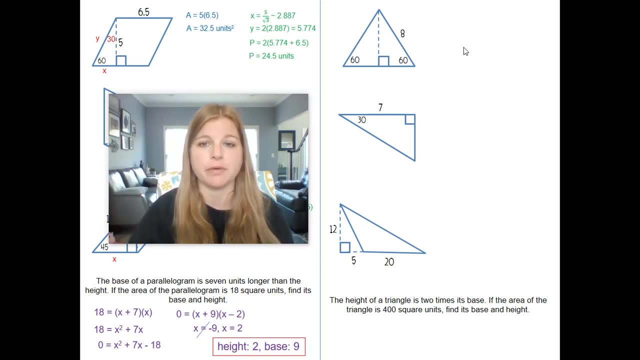 9, because it's 7 units longer, And it makes sense because 2 times 9 is 18.. It all works out. Let's try these problems here. We want to find the area and perimeter triangles. now I need the base and I need the height. I don't have either. I do see that this is a 60,- 60,. 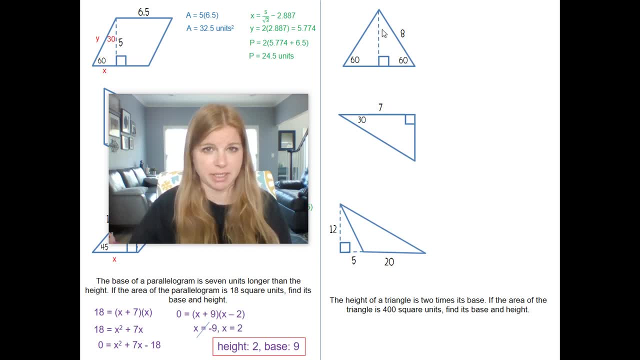 and we have to know that this has to be 60 up here, because if you have two angles that add up to 60, that add up to 120, the third angle would also have to be 60. So it's an equilateral. 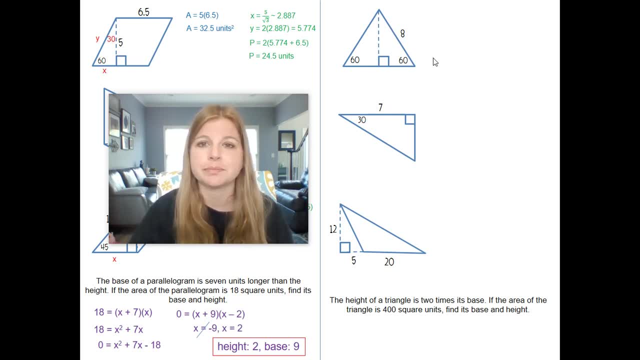 triangle. So keep that in mind for a moment. My 8 is my hypotenuse. We know that if this is a 30,, 60,, 90,, that if this length here, which is opposite the 30, would have to be half, So x would be equal to 4.. If I then want to calculate my y, 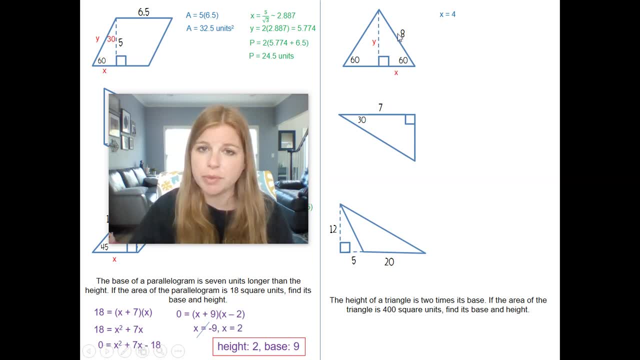 my y is the side opposite the 60. Again, I could do the Pythagorean theorem like I did before, or I could simply take my 4 and multiply by radical 3. I get that 6.928, which we actually. 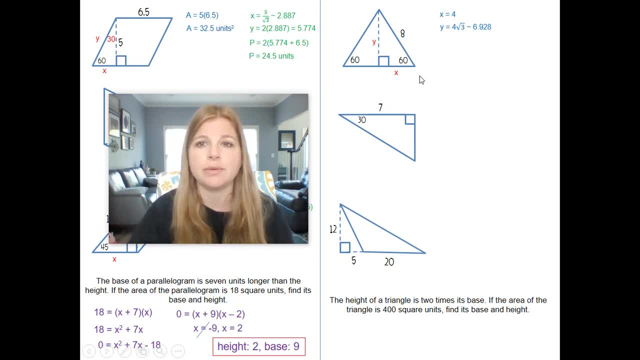 saw in a previous problem. Now that I have that, I know this is 4,. okay, And these are congruent triangles actually, because they have angle, angle, angle side. They're congruent to each other. If this is 4,, then this is also 4.. So my formula: 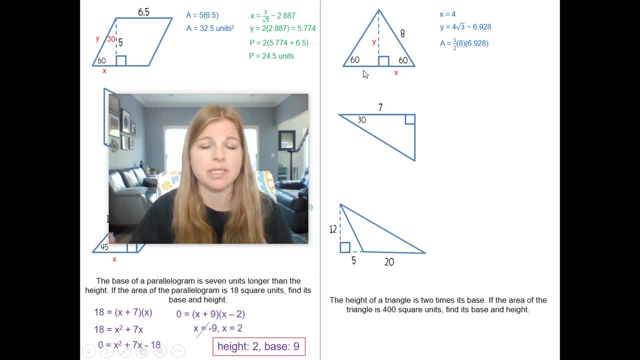 would be 1, half my full base. if this is 4,, then this is 4, 8.. It's also an equilateral, so if this side is 8, then this side would have to be 8, multiplied by my height of that, 6.928,. 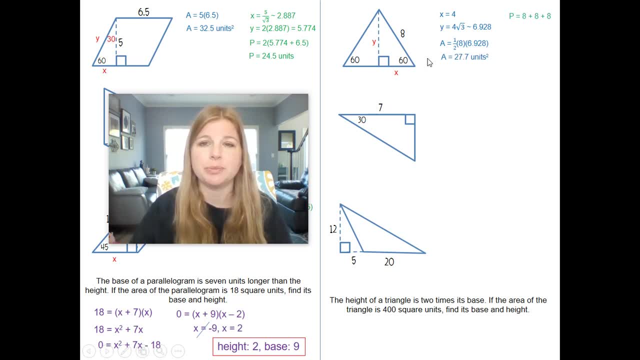 and I get 27.7 units squared. My perimeter is super easy, Since it's equilateral, all the sides would be 8, and I get 24 units. This next one- there's not a lot of information, right, But there actually is. This is a 30-60-90. 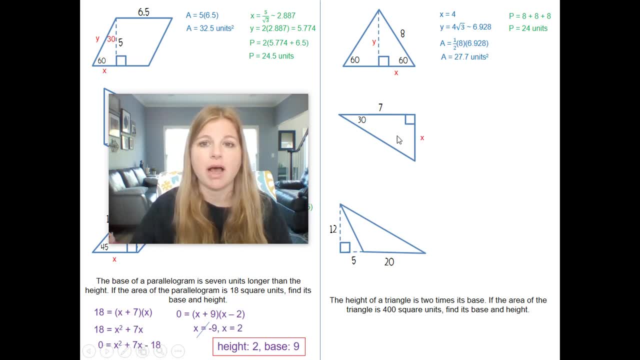 triangle. Side opposite the 60 is 7.. I want to find the side opposite, the 30,, because the 7 is my base. This would be my height. So to find that height I'd have to do 7 and divide it by radical. 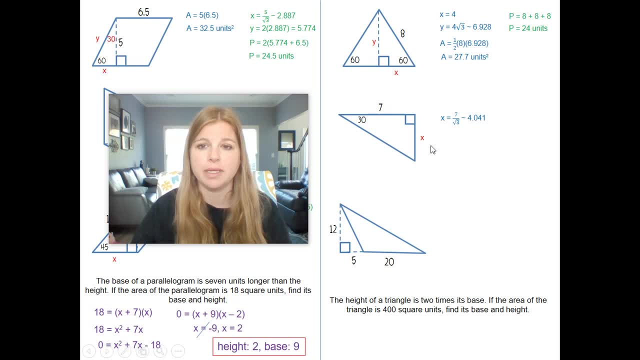 3. I get this number 4.041.. Then I would plug it into my area formula. so it's 1 half my base times my height, We get 14.1 units squared Perimeter. I know this is 7.. I know this is 4.041.. I can simply: 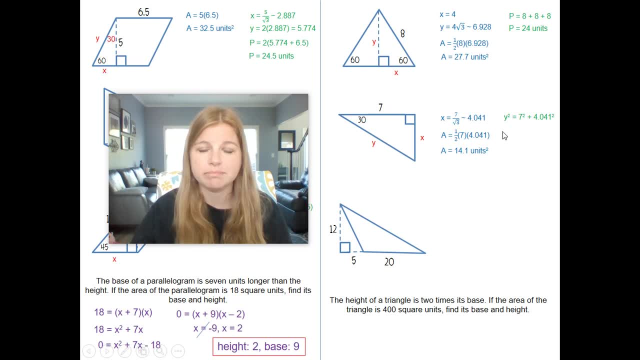 double it to get my hypotenuse. or this is an example of where I could use the Pythagorean theorem. I could say: hey, this is 7.. This is 4.041.. Let me plug it in, or I can just take. 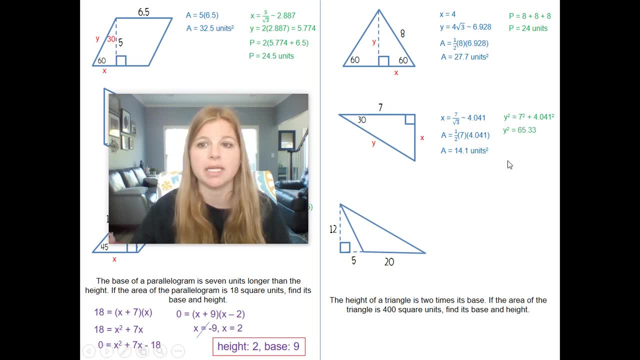 this length of x and simply double it to get the hypotenuse, and I would get the same exact thing. And then for my perimeter it's me simply adding up those three sides: 7 plus 4.041, plus that 8.083.. 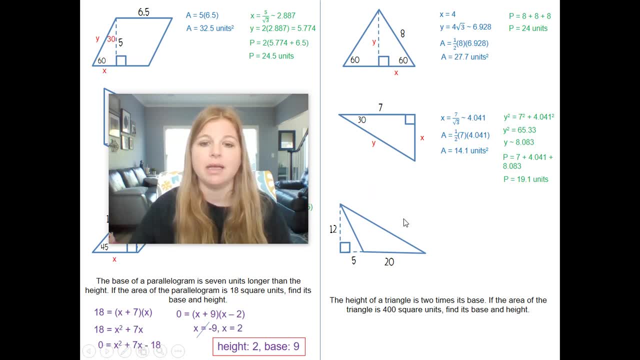 Then we get 19.1 units. Okay Now area formula, Base, times height. So here the base of this obtuse triangle is 20.. What you actually see here is you see that from the obtuse triangle the horizontal has been extended. So you see that from the obtuse triangle the horizontal has been extended. 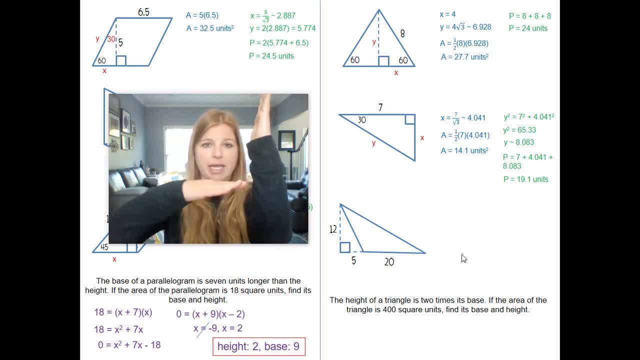 And then a vertical has been created to get a 90 degree angle. The purpose of that is so you can actually see what the height of the triangle is. The height of the triangle is 12. So it goes that many units up, But the base is not from the right angle. It's just what you actually see for the 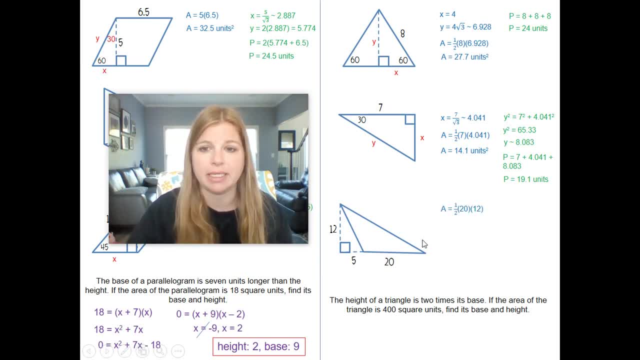 triangle 20. So I actually have my base and height here. So it's one half base of 20 times the height of 12. And that ends up being a pretty easy problem. It ends up being a 120 units squared. But perimeter is a different story, Because the only side of this triangle 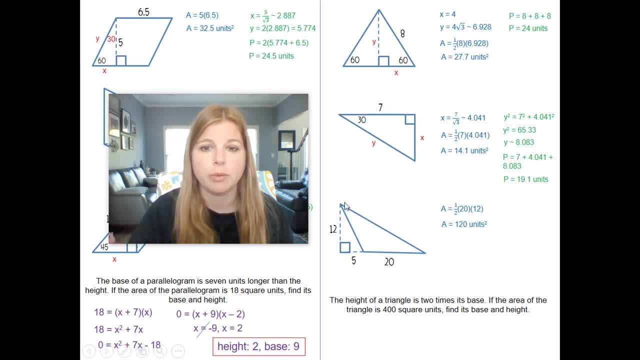 that we actually know, for perimeter reasons, is this 20.. We don't know this length. We don't know this length, But because this right angle is here, that helped us with the height, this now helps us create use the Pythagorean theorem rather, as we don't see any 30 or 60s, We can't 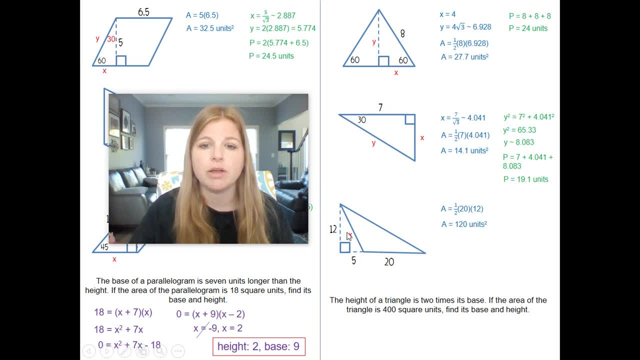 determine that We can't assume it if we don't see it. So if I wanted to find this length here of the triangle, notice this is the hypotenuse Of this triangle here, this right triangle. So 5 squared plus 12 squared would be equal to x. 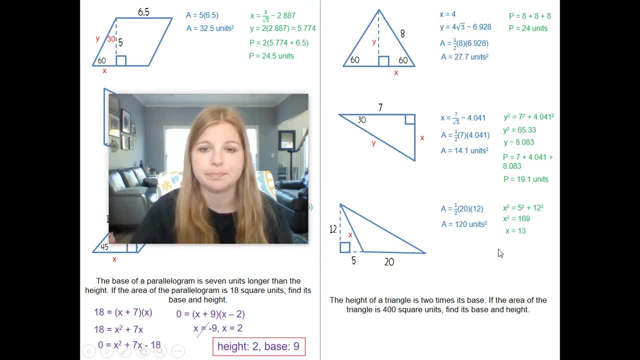 squared, which ends up giving us 13,, which is nice. And now, if I wanted to find this hypotenuse of the big triangle including this right angle here, it would be: 12 squared plus 25 squared equals y squared, which ends up giving me about 27.731.. Now that I have my three sides, I know. 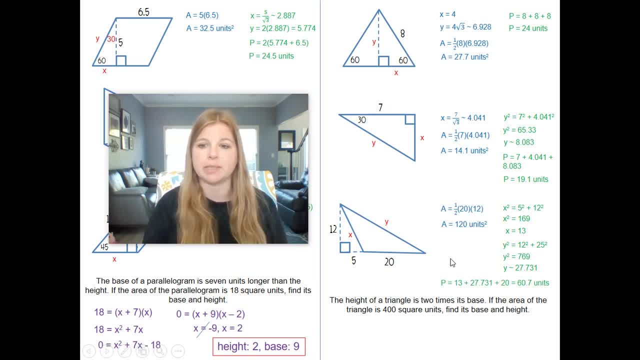 what x and y are. I can add those up and I get my perimeter. So from here we're going to do that. So first of all, let's clarify this element of the Postmodern version of the front triangle to using that to do that to. 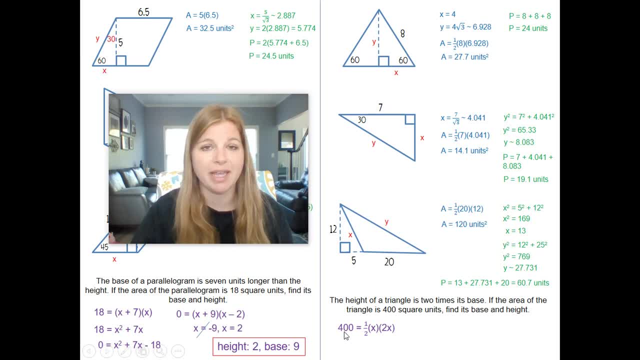 find out what the actual area of the triangle is moving through. the says at block here. So, guys, if we're going to do our best to find out what the area of the triangle is moving through at 4 squared, this is where I'm going to do that. 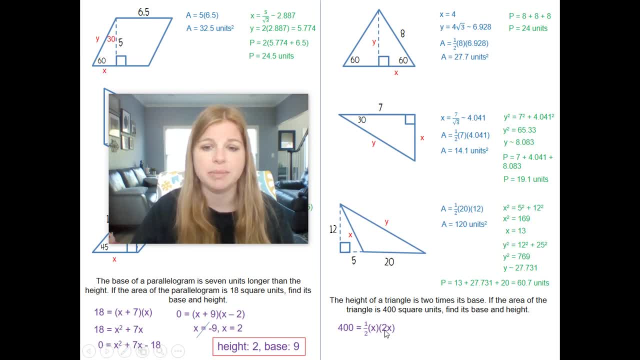 And it's going to be HomayoutthOW and I'm going to do this sort of a bony type content rather with this: All right, half of 2 is 1.. So this is really just saying 400 equals x squared. Square root of 400 is 20.. 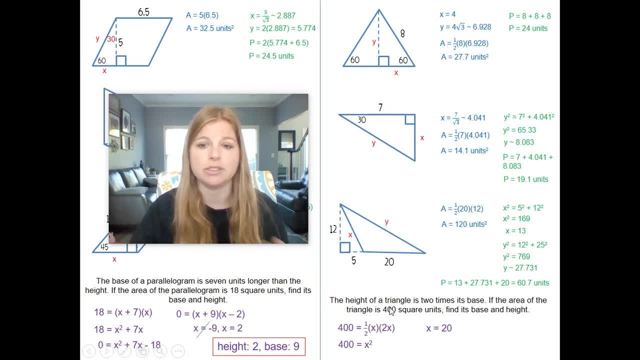 So that would mean my 20 is my base. The height is 2 times the base, So the height would be 40. And it makes sense. If I multiply 40 and 20 together I get 800.. Take half of it, It brings. 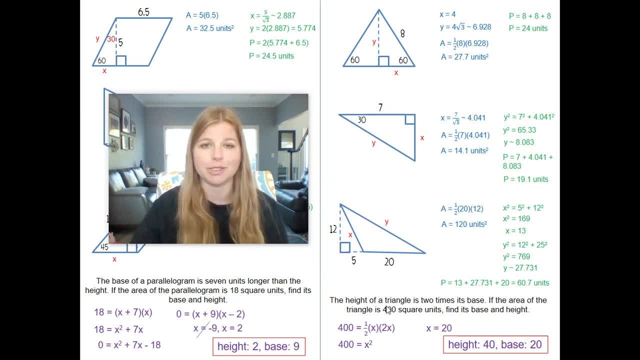 me to that 400.. I hope this video was helpful for you. Thank you so much for watching Bye.